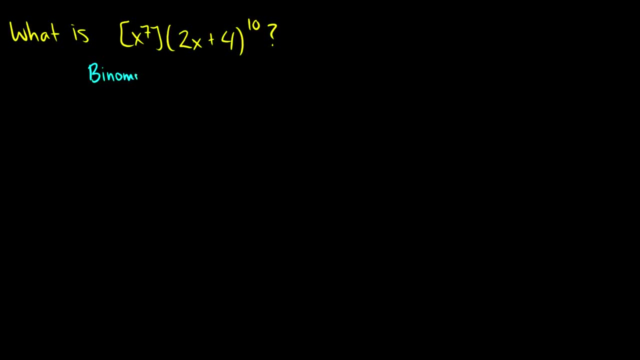 theorem. Of course you'll remember this from the first Discrete Math course, And if you don't remember, x plus y to the n is the sum of i equals 0 to n of x plus y to the n. So we have n choose. i times x to the i, y to the n minus i. So a little bit complicated, but 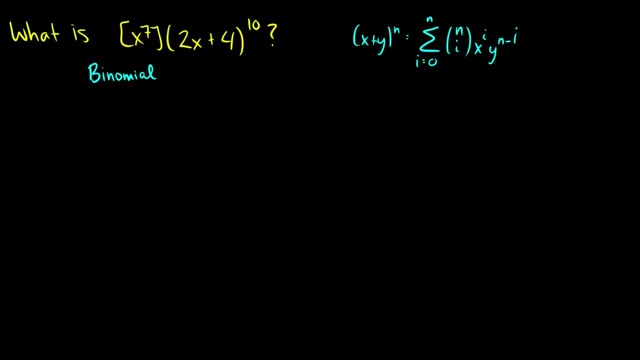 we'll see it in action here. So we want x to the 7.. So what this really means is that we want 10, choose 7.. We want 2 times x to the 7, which means that this y value 4 is going. 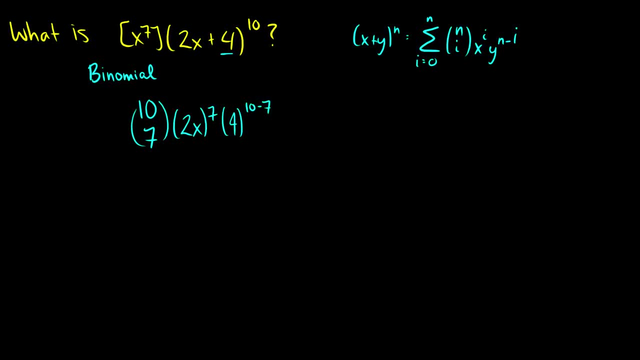 to be to the 10 minus 7.. Subtitles by the Amaraorg community, which is the same thing as 4 to the 3. So I'm not going to simplify it really anymore, but essentially what we've done here is we've taken our x and this is our y, and because 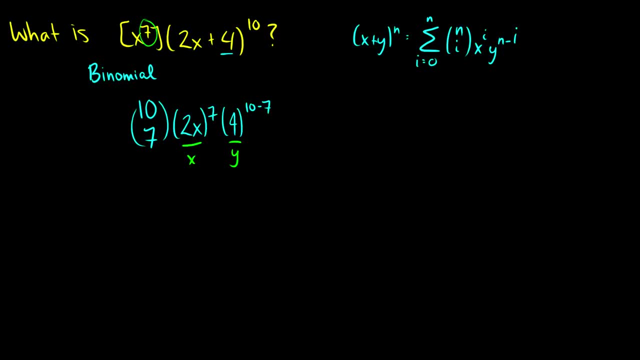 we're looking at the 7th power. of course, we want our x to have the 7th power and we should be choosing the 7th power as well, which is denoted up here in this sum as n choose i x to the i, So that is the coefficient of x to the 7.. So you've kind of done this before. 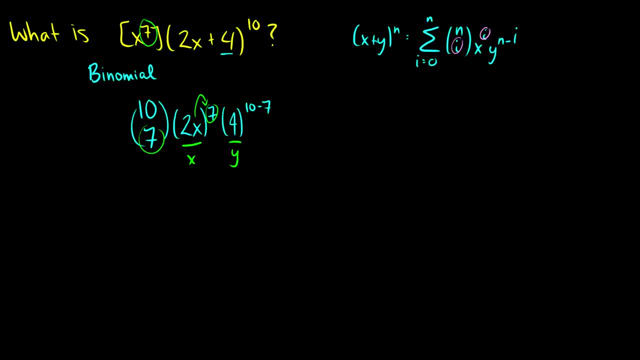 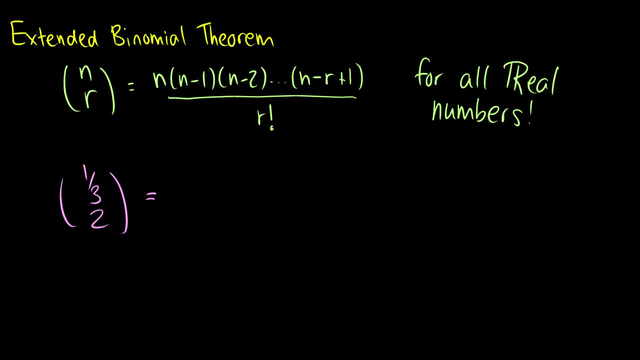 but just not. maybe with this notation. Of course, we can make things a little bit more challenging, but before we do that, I need to teach you this extended binomial theorem, otherwise you won't be able to find out some of the more difficult coefficients. So we've used 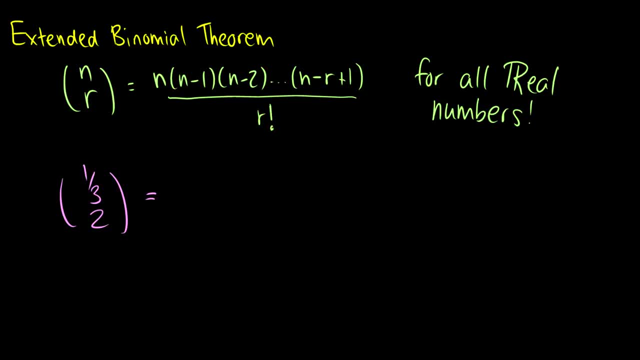 the definition n choose r. So we've got 4 to be n factorial over r factorial, times n minus r factorial, and that works. but the problem is that it assumes this is a real, an integer, a positive integer. but we can use the binomial theorem for more abstract things like: what is a third choose? 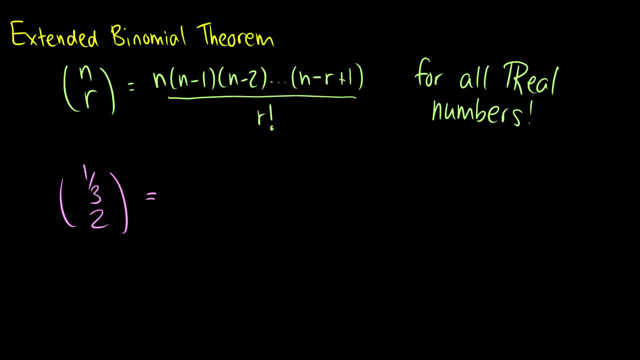 2.. Well, we need to use this definition up here, which is n times n minus 1 times n minus 2, all the way down to n minus r plus 1, all over r factorial. You can see this follows from this definition here. So what we're doing is: I want to get rid of this n minus r factorial. 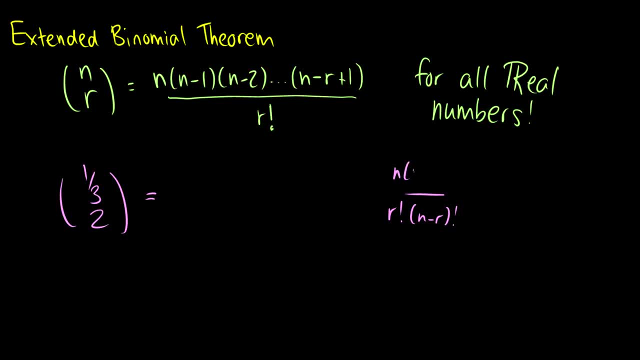 at the bottom. So what I do is I just expand n all the way out until I get to n minus r plus 1 and then n minus r- factorial, And then I just cancel it here. So this follows from the old definition, and what's cool is: 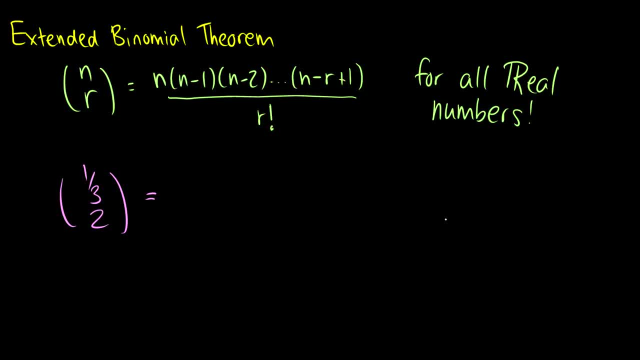 that we can put in any number we want now. So let's do one third, choose 2.. So we have one third times. well, we want one third minus 1 now, And we only wanted two terms. so that's good for the top. 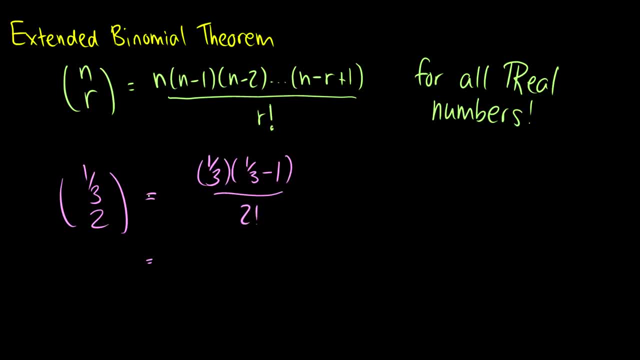 And we're choosing 2.. So it's over 2 factorial. So this is just going to be one third times negative, 2 thirds over 2 factorial, which is the same as negative 2 over 9, all over 2 factorial. So this is: 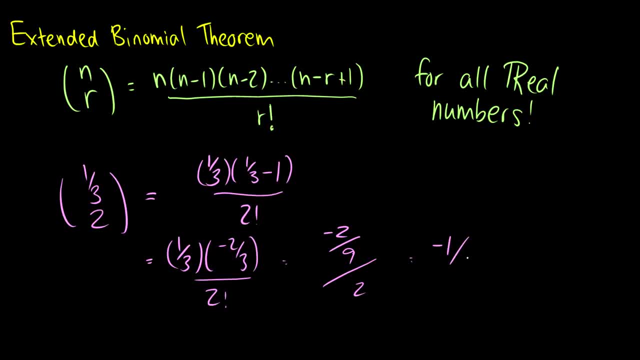 going to be negative: 1 over 9.. So one third choose 2 is negative 1. ninths, and you're saying: hold on a second. you can't choose 2 over a third of an object. You are right. You're absolutely right. 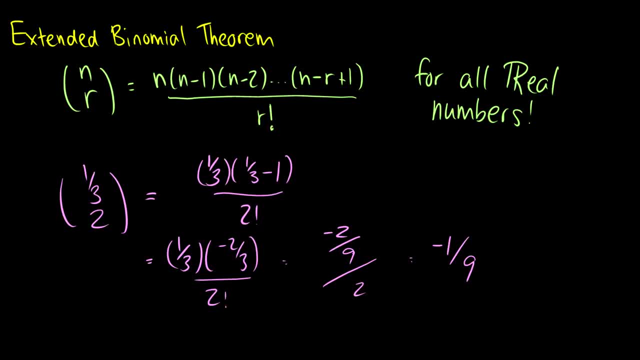 But it's a little bit more abstract. You know you can't choose 2 out of a third, So this is one of those things that follows mathematically and works absolutely properly but might not make intuitive sense. So understand the abstraction behind it and you'll see its use in just a 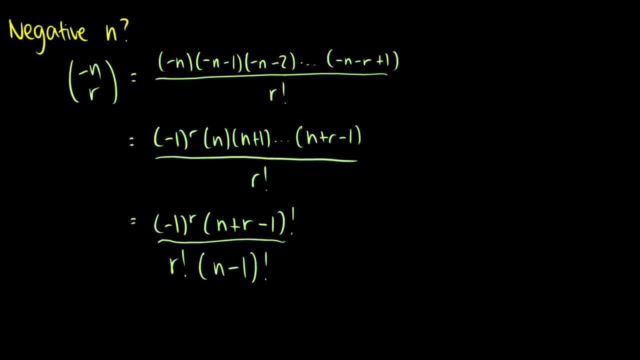 few moments, But first we can do it for negative numbers too. So here's where it even gets easier. What does negative 6 choose? 2?. Hold on a second. Do you want to choose 2 objects out of negative 6?? 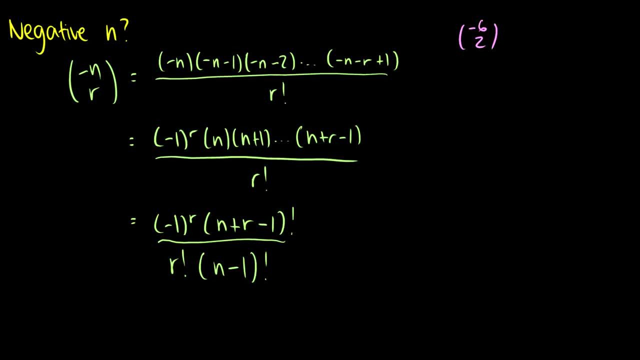 Are you crazy? What do you mean? choose 2 objects out of negative 6? You can't do that. Well, with our definition of the expansion of the n choose r operator, we can. So I've written out a few steps here. I'll go through this. 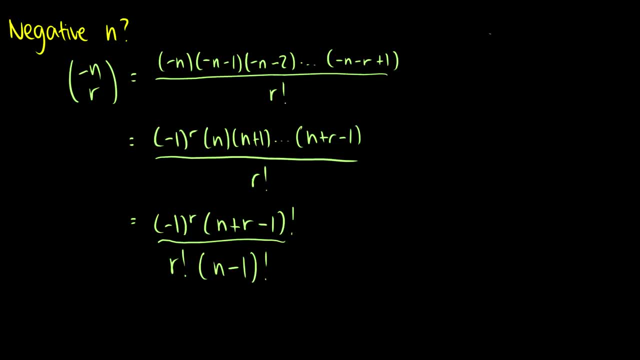 So in the first step we start out with negative n. We go all the way down to negative n minus r, plus 1, all over r factorial. This is the same as the previous example. Then what we do is we factor out a negative 1 from each of these terms. 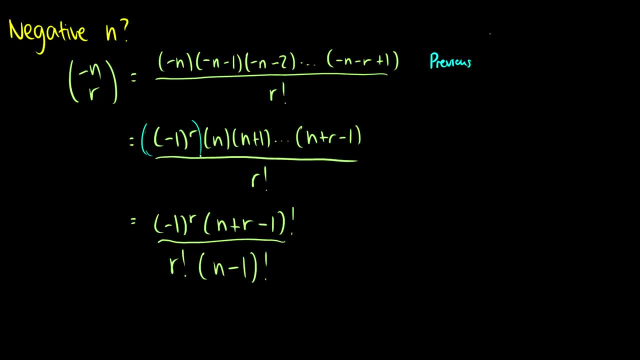 So we get a negative 1 to the r here, Just like we did. Well, not just like we did, but because there's r terms, Because we're choosing r terms, we can factor out negative 1 r times. So we get negative 1 to the r. 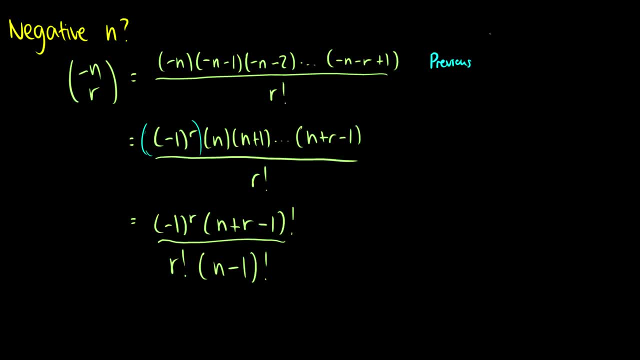 And then what we do Is we just kind of reverse the step we did in the last page And we change this to n plus r minus 1- factorial Notice it only goes down to n. So it's n plus r minus 1 all the way down to n. 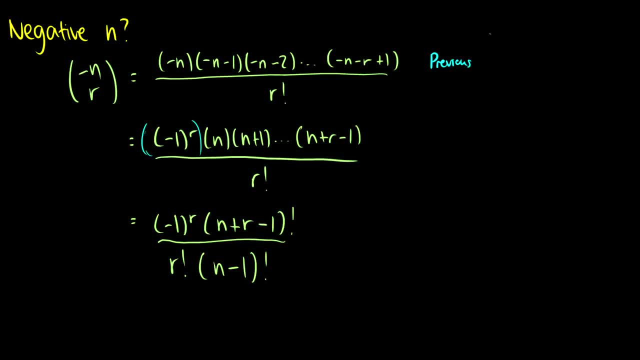 So we have to sort of add in this n minus 1 factorial on the top and the bottom to cancel out And we end up with this result at the bottom here. So negative n choose r is just negative 1 to the r times n plus r minus 1.. 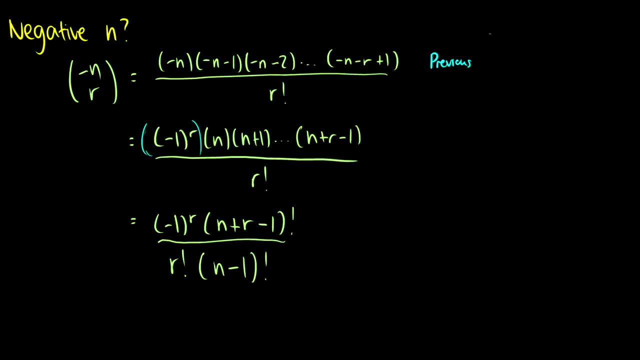 Over r. factorial times: n minus 1. factorial, Which simplifies to: n plus r minus 1 choose r. times negative: 1 to the r, Because this is just the definition of n plus r minus 1 choose r. So what's interesting is that when we have a negative n, 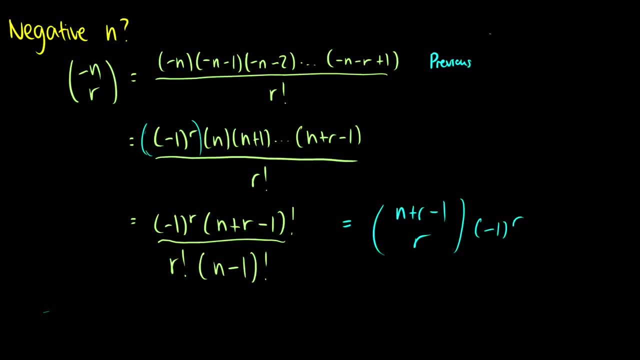 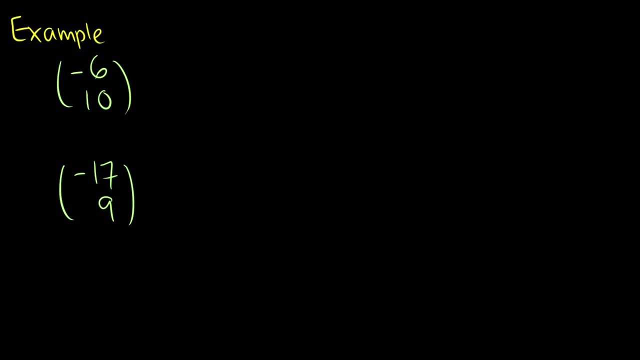 We end up with the combinations, with repetition formula, With, of course, this negative 1 to the r, Which depends whether it's positive or sorry, even or odd. But it's kind of an interesting result. So let's do a couple examples. Well, I'm going to leave this formula over here on the side. 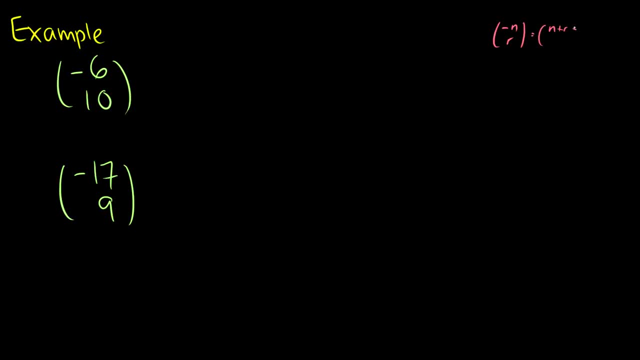 Negative n. choose r is equal to n plus r minus 1. choose r times negative 1 to the r, Because I think it's more important To be able to do these quickly Than it is to write out every single step. So we know that this is just going to equal. 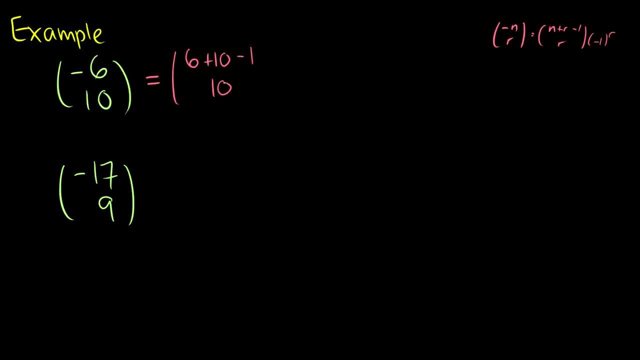 6 plus 10 minus 1 choose 10 times negative 1 to the 10.. So this is just going to be 15 choose 10.. So negative 6 choose 10 is just the same thing as saying 15 choose 10.. 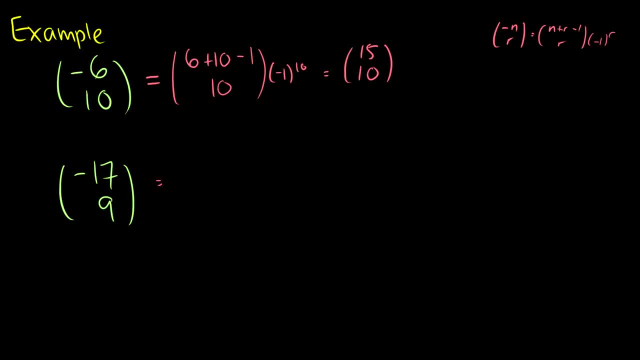 What about negative 17 choose 9.. Well, this is going to be 17 plus 10 minus 1, choose 9.. Sorry, that should be plus 9 minus 1.. Then we get negative 1 to the 9.. So we're going to get negative. 17 plus 9 is 26 minus 1 is 25, choose 9.. 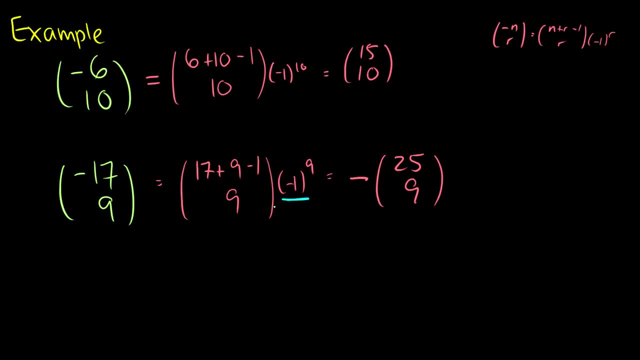 And, of course, this negative comes from the fact that we have an odd r value, So pretty simple actually to do negative expansions. It's kind of interesting, I think, And the question is, why do we need to know this? Why do we need to have the extended binomial theorem to include negatives? 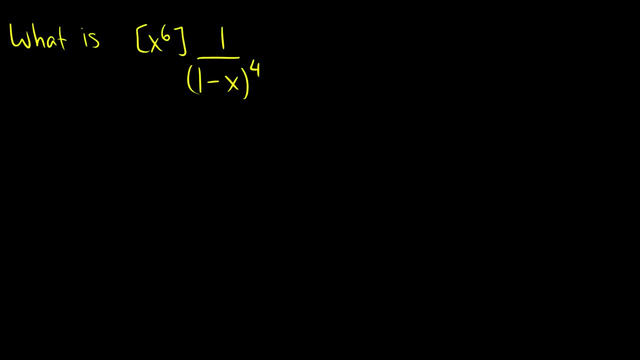 Well, here's why I want the coefficient of 1 over 1, minus x, to the 4.. Now, how do we do that? Because we're dealing with Negative x is here. So, first of all, we can rewrite this, We can make this a little bit nicer. 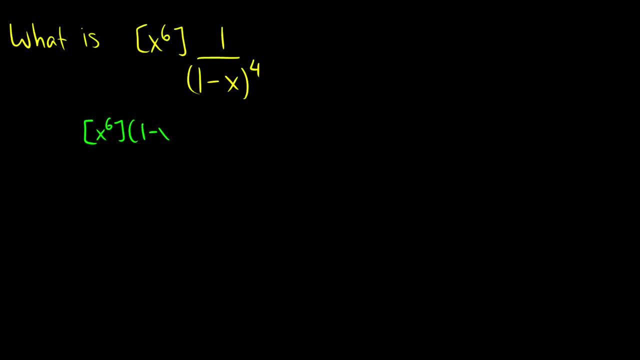 So this is x to the 6 of 1 minus x to the negative 4.. Okay, So when we have this example, This value right here is our n And this value right here is our r. Now, why is it this way? 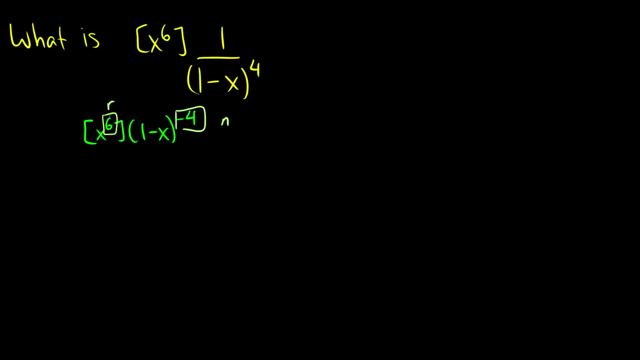 Well, we have negative 4.. And we're choosing 6 of them. So this x to the 6 is actually equal to negative 4: choose 6.. And, of course, because we're dealing with this negative x here as well, Because we're using the binomial theorem. 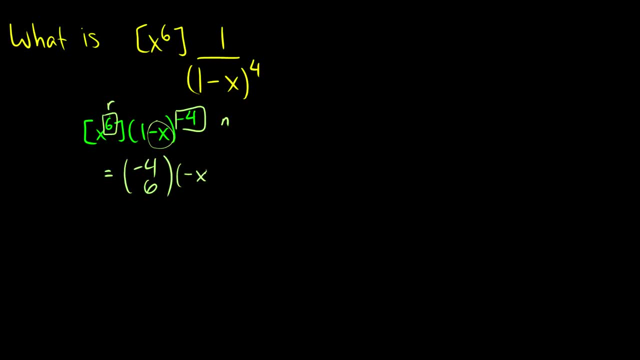 We have to include this negative x to the 6 as well, Because we're choosing negative x or 6 negative x's. So what happens here Is, with the expansion, before We get 4 plus 6 minus 1, choose 6.. 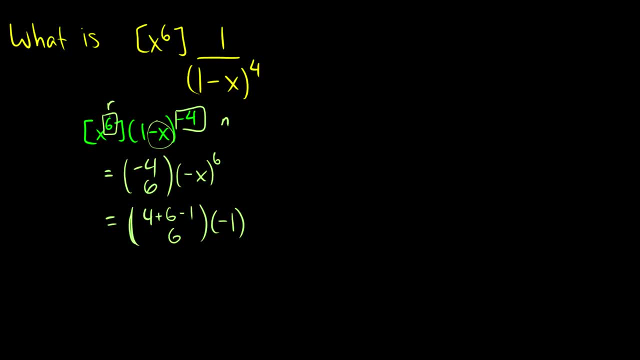 Times negative 1 to the 6. Because of our expansion. And we'll split up this negative x here, And we'll split it into negative 1 to the 6 times x to the 6.. Well, because we're looking at only the coefficient. 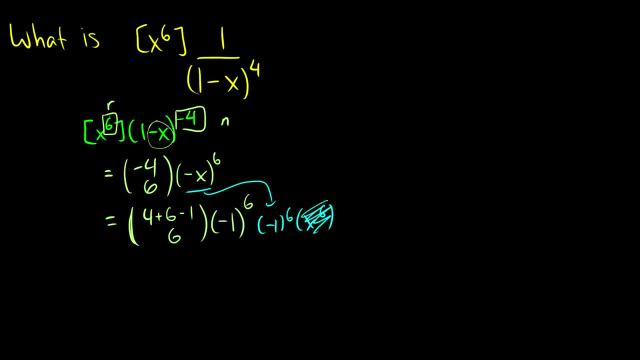 We really don't need this x to the 6 here. That's not really important, And you'll also see That we have a negative 1 and a negative 1 canceling each other, Because a negative times a negative is a positive. 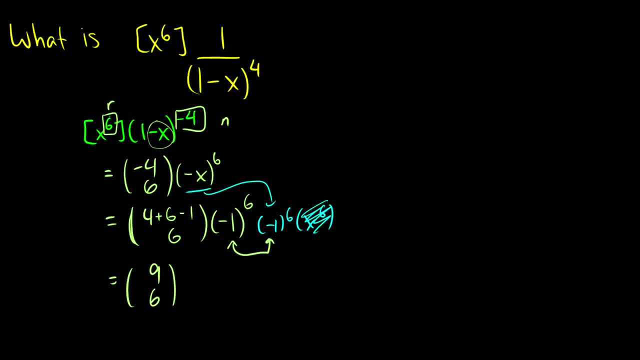 So our end result really is just 9, choose 6.. So the coefficient of x to the 6 in 1 over 1 minus x to the 4. Is just 9, choose 6.. So if you ever have a 1 minus x on the bottom, 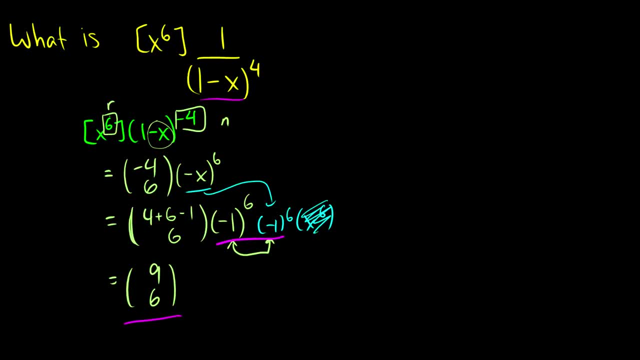 Your answer is always going to be positive, Because your negative 1's will cancel out. It's kind of cool. So that was a fairly straight forward one, I would say, And let's make it a little bit harder. Okay, what is the coefficient of x to the 8.. 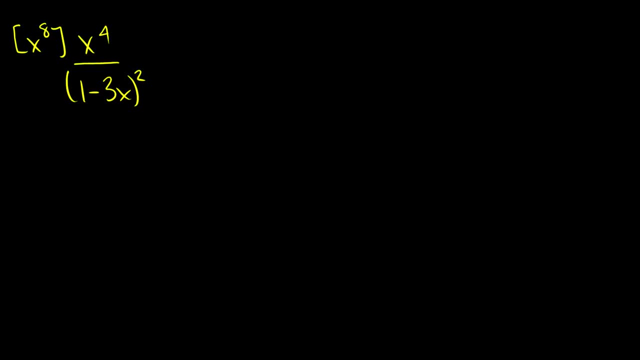 Of x to the 4th over 1 minus 3x squared. Okay. well, How do we deal it with When we have this x to the 4 on top? Well, Here's the thing We've kind of just shifted. 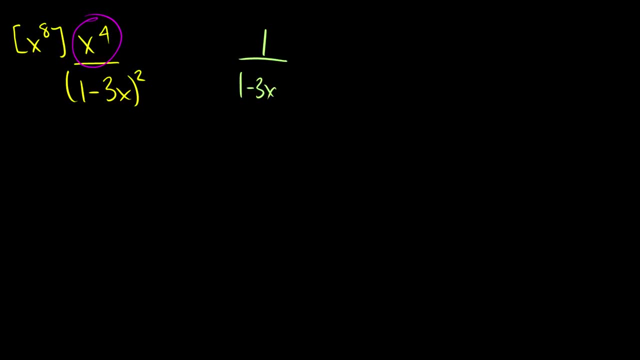 This 1 over 1 minus 3x squared function. We've sort of just shifted it over By x to the 4.. So We can rewrite this As actually just saying: What is the 4th coefficient Of 1 over 1 minus? 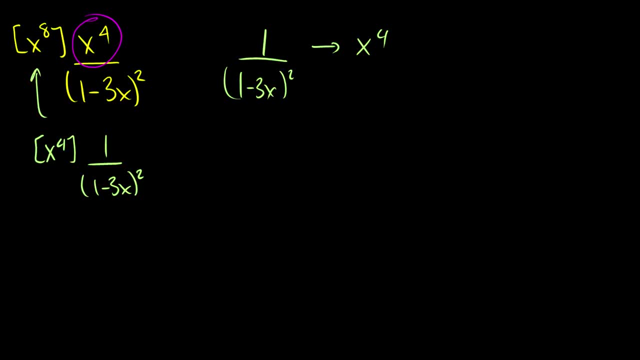 3x squared. You're saying: hold on a second. Why does this work? Well, think of it as saying: well, Every term is going to be shifted over By x to the 4.. So we're multiplying the whole function By x to the 4.. 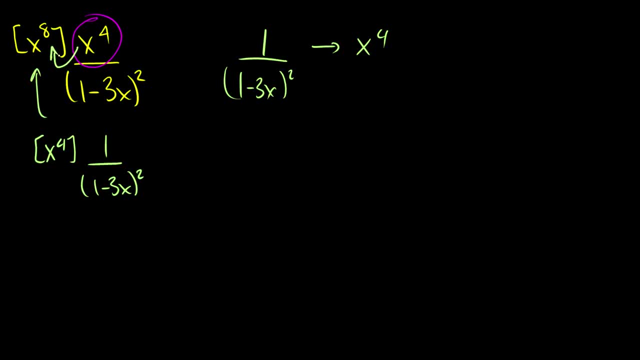 So Why don't we just Put that x to the 4 back into x to the 8. And see what we have left? So that's what we did. Now we want the 4th coefficient Of 1 over 1 minus 3x squared. 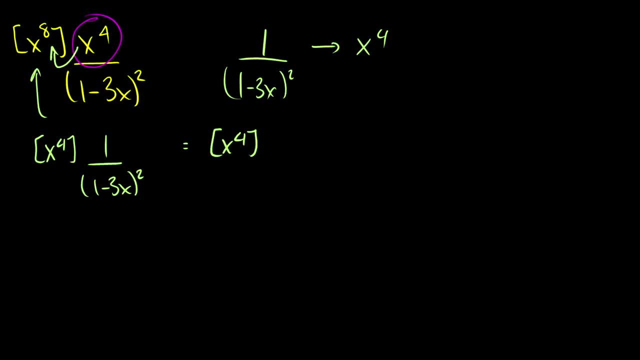 Well, again, we can rewrite this A little bit nicer. So this is going to be 1 minus 3x To the negative 2. And again, we have an n value here. We have an r value here, So let's plug those in. 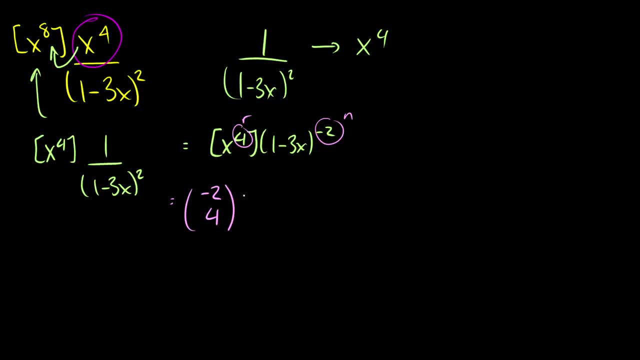 This is negative 2, choose 4.. Of negative 3x To the 4.. And we can expand this, So this will be 2 plus 4 minus 1, choose 4.. Times negative 1 to the 4.. 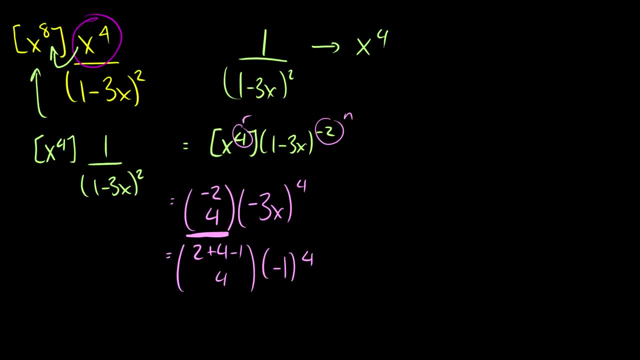 And that is the expansion of negative 2, choose 4.. Now we'll expand negative 3x to the 4.. This is just going to be Negative 3 to the 4. And we don't need the x to the 4.. 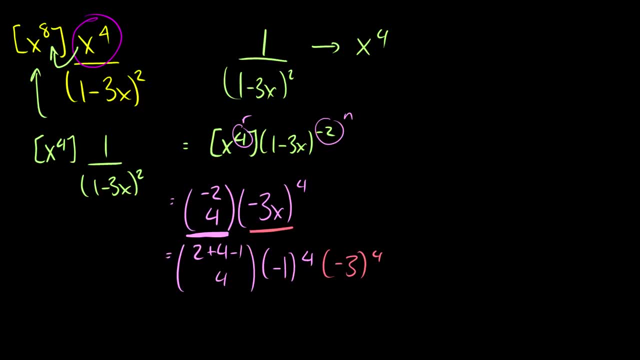 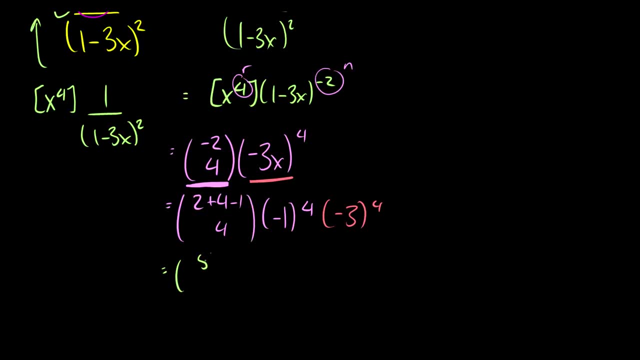 Because we're only looking at the coefficient, So We get our result As 5 choose 4.. This negative 1 and negative 3. They'll end up becoming positive, So this is really just 5 choose 4.. 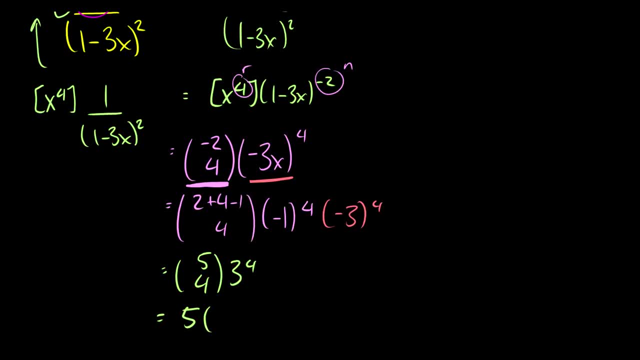 Times 3 to the 4. Which we know is just 5 times 81. So we can actually compute that, Which we know is a 405.. So What this says Is that If we take x to the 4.. 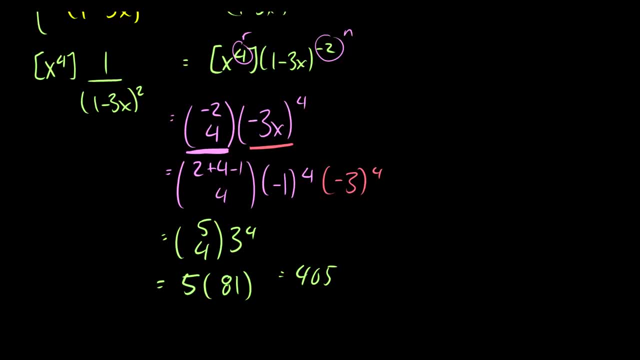 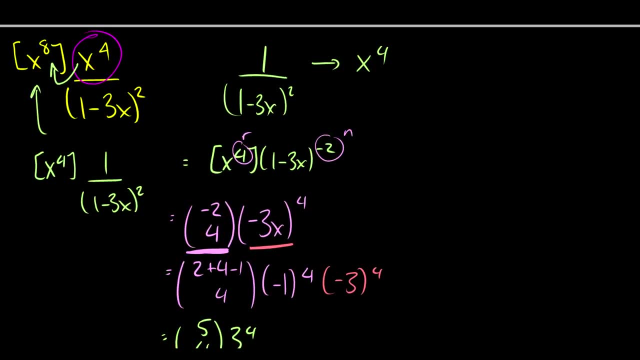 Of 1 minus 3x squared, We'll get 405.. So When we shift everything over By 4 values, It'll be the 8th Coefficient of x to the 4. Over 1 minus 3x squared. 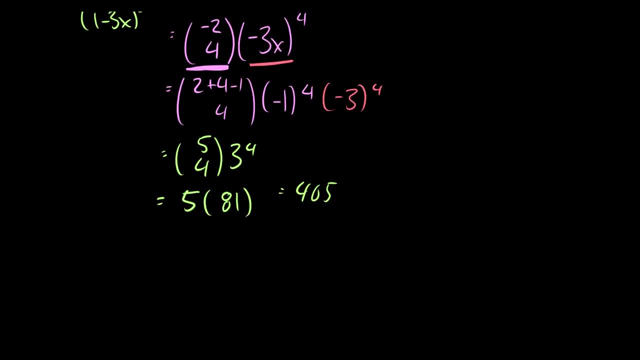 So that's a little bit more of a tricky example. Of course you can plug these equations into Wolfram Alpha And you can check for yourself that these are indeed the coefficients. So that's a nice way you can check. You can just plug the function right in. 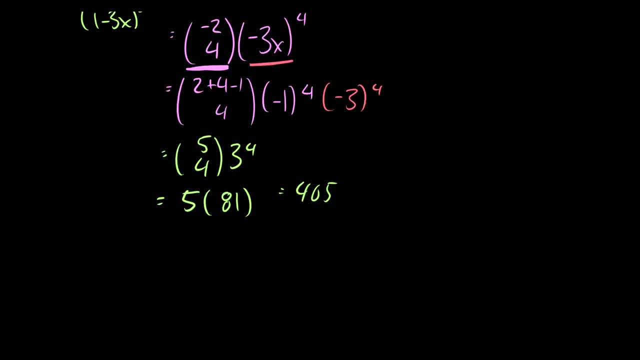 And you can search for that x value And that's a great way to check your answers. Let's do A word problem. These are fun. If a fair die is rolled 12 times, How many ways can they sum up to 30?? 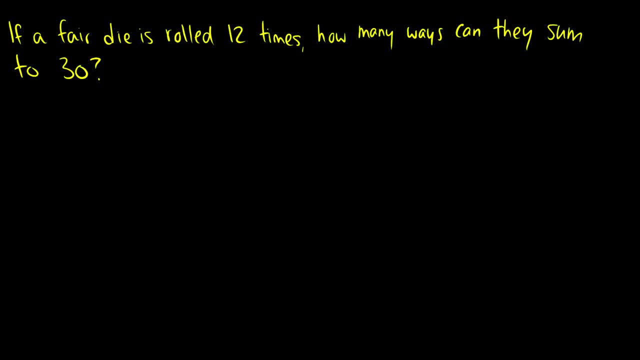 Okay. so We need to think about this a bit. We want them to sum up to 30. So we're going to want The 30th coefficient Of some equation. And what's the equation? Well, For a die. 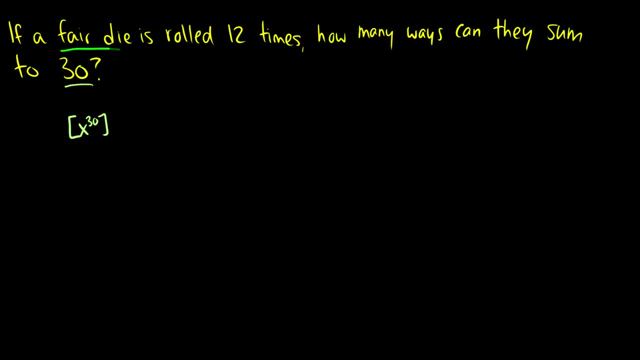 This is going to have 6 sides In this question, So It's a 6 sided die. So What are the options? The options are going to be 1., 2., 3., 4., 5.. 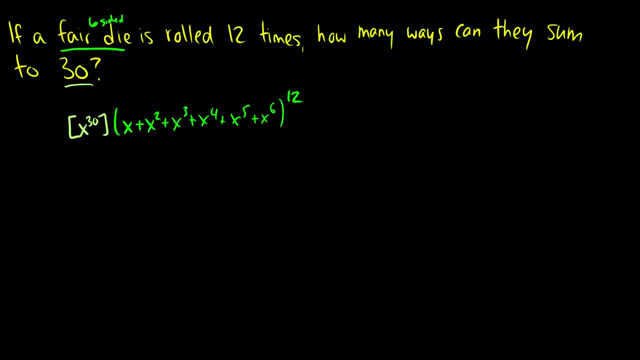 And 6. And we rolled this 12 times. So We'll pick one of these Each time for 12 rolls. So What do we do here? Okay, well, X, 30 of X plus X squared, plus X cubed. 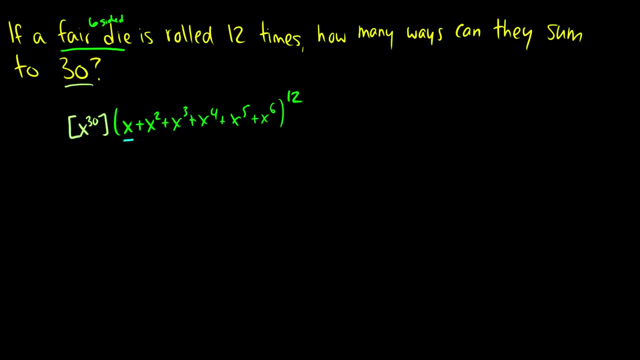 We need to factor out An X out of all of these Because we want Our generating function to start at 1.. So we'll just take an X out. So this will be X 30. Of. We're going to take an X out of the first one. 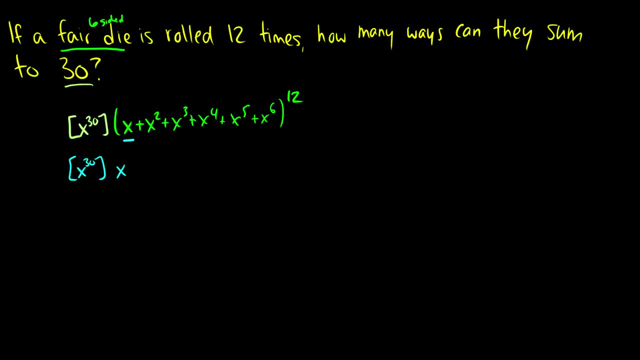 We're going to take an X out of the second one Out of the third one Out of the fourth one, And so on. So we're going to take 12 X's out Over the course of this. This will be X to the 30th coefficient of X: 12.. 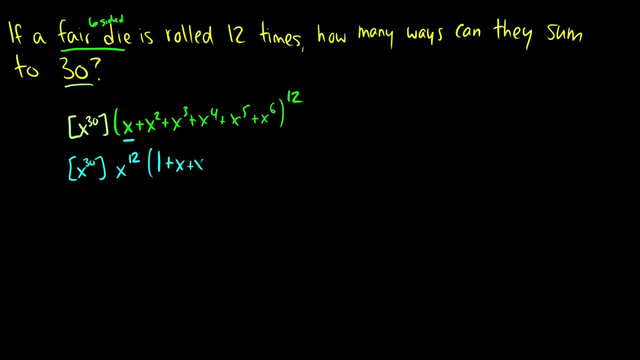 Times: 1. Plus X Plus X squared. Plus X, cubed. Plus X fourth. Plus X to the fifth. All to the twelfth. We'll do what we did in the last equation And we'll just Shift it over. 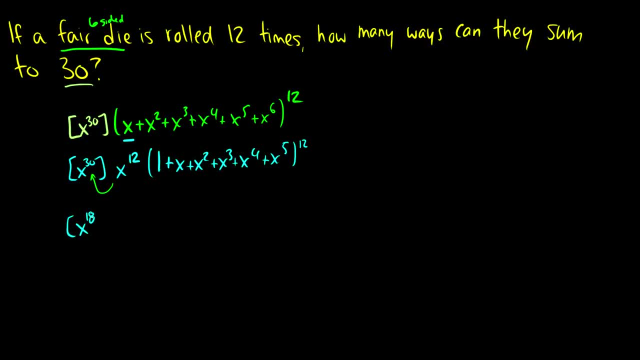 So really, what we're looking at here Is X to the 18.. Of One plus X Plus X, squared All the way up to X to the five, Raised to the 12th power. Now things get a little bit trickier. 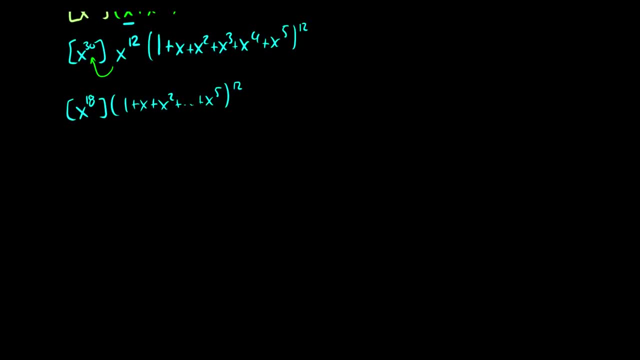 Because what is this generating function? Well, This is, Of course, the 18th coefficient of One minus X to the sixth Over one minus X. This was talked about in the previous video, So if you can't see this, Please refer back to that one. 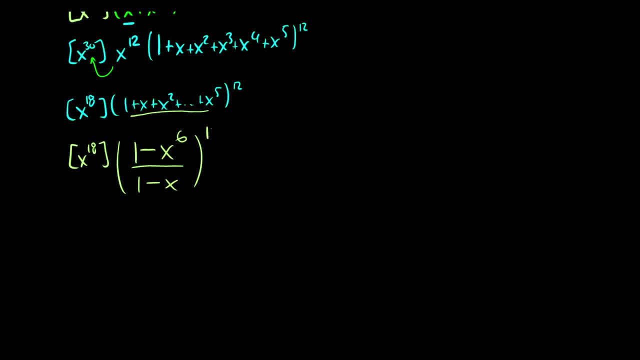 And this is raised to the 12th power. Okay, So let's write this a little bit nicer. This is X to the 18.. Of One minus X to the sixth, All to the twelfth Times, One minus X. 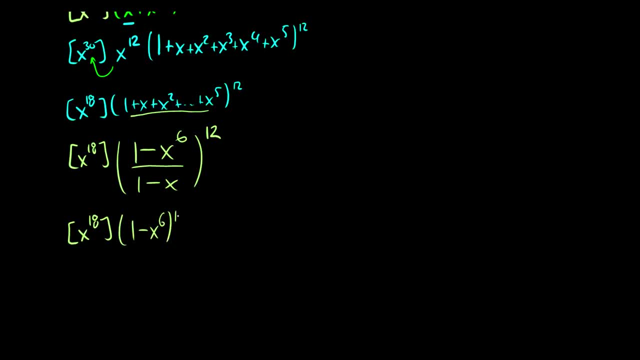 To the negative 12. This is where things get tricky, In fact, It's where it gets very tricky, So Listen up very closely to this. I had Troubles With this. This is where things get tricky, In fact. 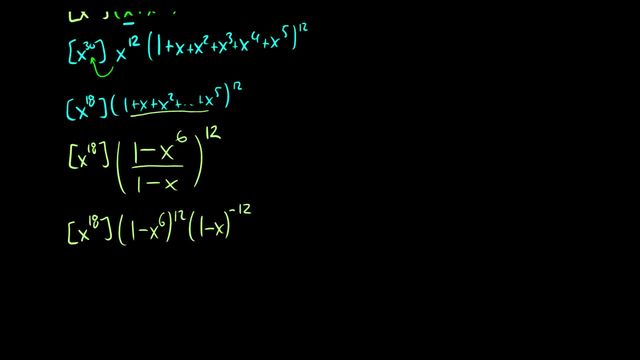 It's where it gets Very Tricky, So Listen up very closely to this. I had Troubles With this For quite a while, Never really understood it, Until I got to my final exam In the course. 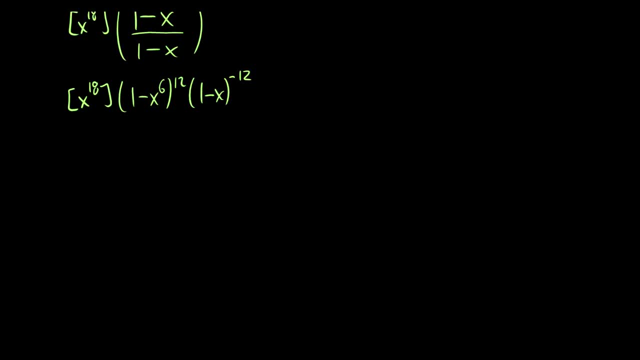 And it wasn't even used there. So How disappointing, Right, But We need It to sum To 18.. So These are two different binomial expansions. One is a negative 12.. One is a 12.. 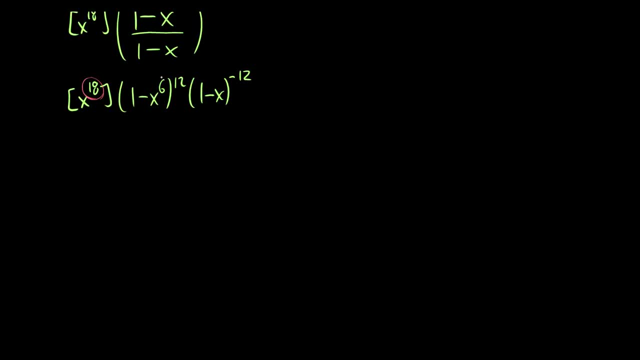 We need to choose 18 total. So What we want Is All possible combinations. So What we want Is All possible combinations. So What we want Is All possible combinations. So Let's suppose We have different cases here. 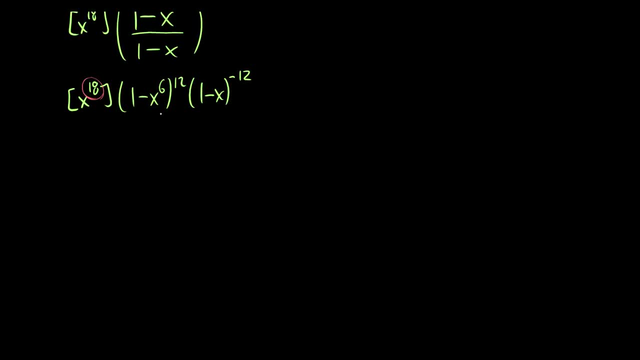 Because we need different cases, to do this. In the first case, In the first section, We have 12 as our n. We're going to choose 0. Of the x to the 6's, Which means That we have to choose 18.. 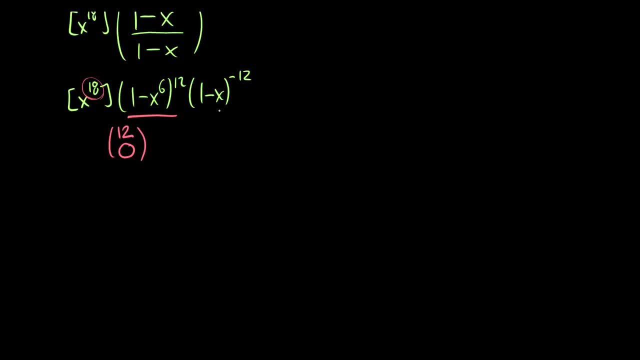 Out of the second part here, So This will be On blue, So We're going to choose 18.. Out of the second part here, So This will be On blue, So We're going to choose. 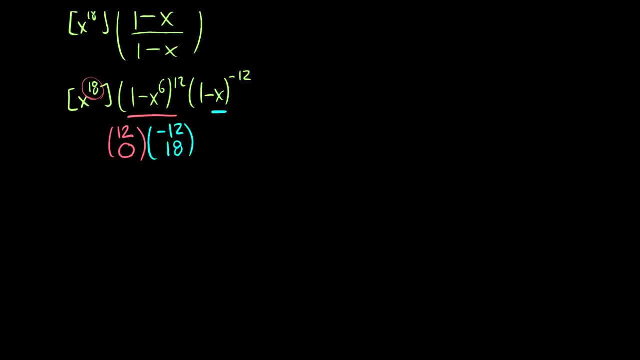 18. Out of negative 12. Because We don't have any x6's And we have to get up to x18. So we have to choose 18. Of the x1's Now, What about the case? 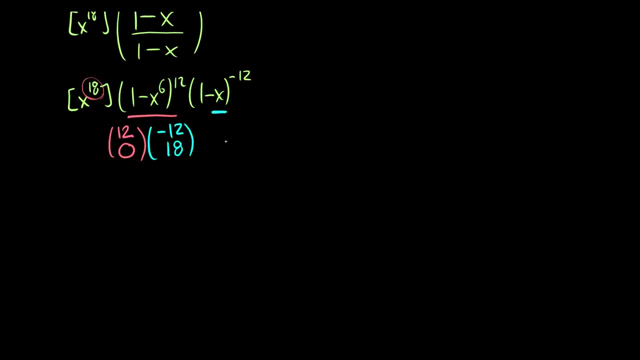 Where we choose 1. Of the x6's. So Let's 12 choose 1.. And If we have x6. Then that means We have to choose 12. Out of the x1's. So 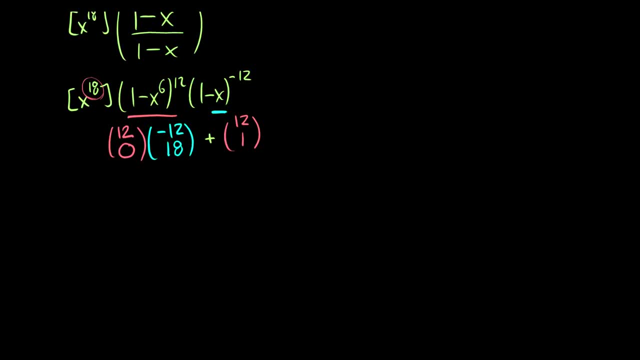 This will be 12.. Out of the x1's, So This will be 12.. Out of the x1's, So This will be 12.. So This will be Negative: 12. Choose 12.. 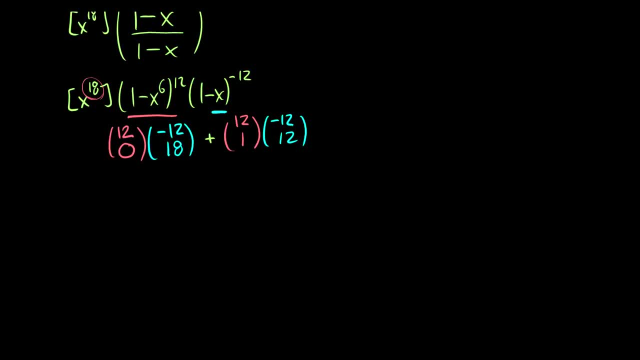 And What also should be noted here Is that, because I'm only choosing 1 of the x6's, When I expand it I'm going to get a negative 1. Times x to the 6 here, Because This is a negative number. 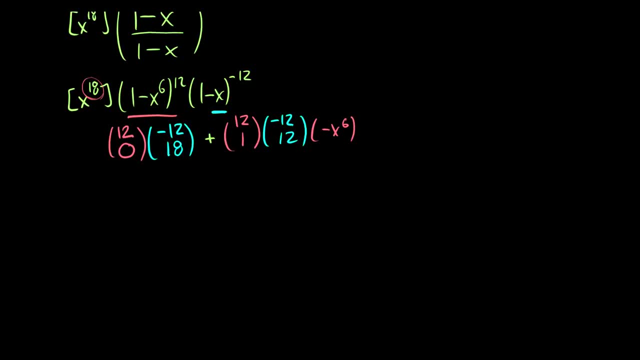 Negative x to the 6th And I'm choosing 1.. So my answer is going to be multiplied by negative 1. So Put that Negative 1 there. Let's add The next part. Suppose I choose 2.. 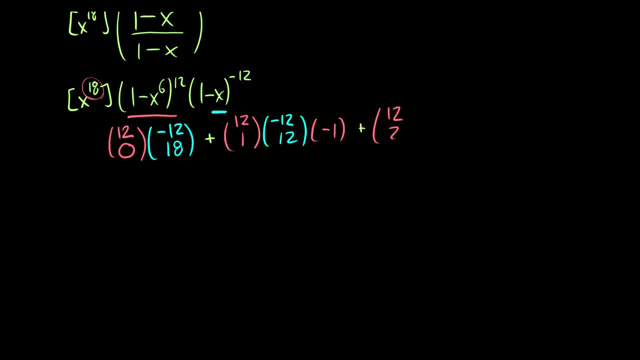 x6's, So 12.. Choose 2 of those. Okay, So I have x to the 12 now. So I have to choose 6 more Of the x1's, So It will be Negative 12.. 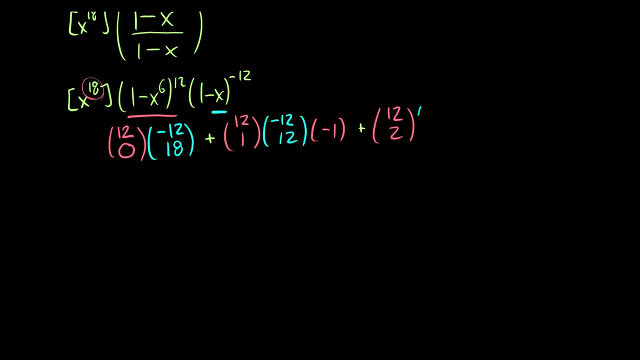 Choose 6. And then our last case: Well, Suppose I choose All 3. x6's, So This will be Negative. 12. Choose 6. And then our last case: Well, x6's, Of course. 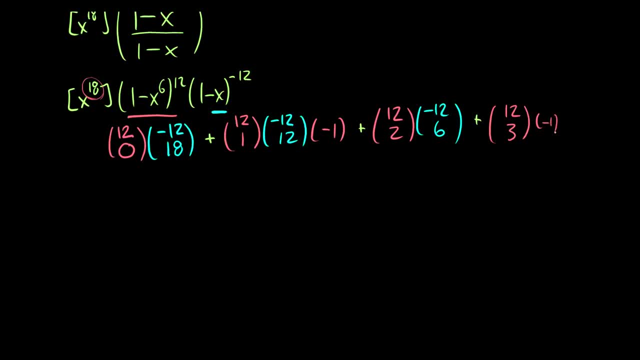 It's going to be Negative. 1. Because we're choosing 3 negative numbers And That means That we can't choose Any Of the x1's, So It will be Negative 12. Choose. 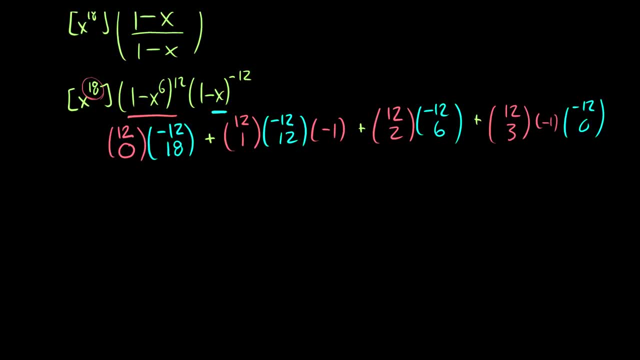 0.. So These are all the cases We have And It's Amazing, Right, Because There's. You know, You're multiplying 2 numbers, So you think You can Multiply a bunch of things. 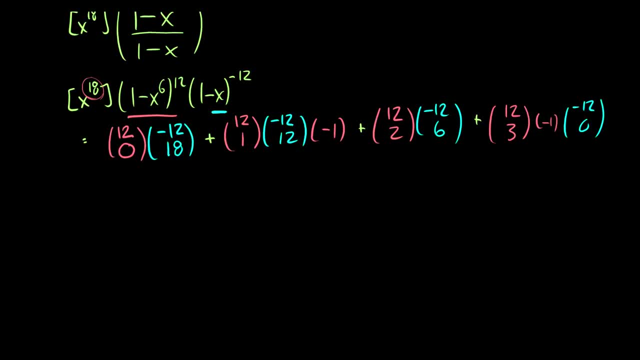 But you have to consider All the cases where, Okay, We choose 1 out of the first one, We choose 2 out of the first one, 3 out of the first one. I could choose 4 out of the first one. now, 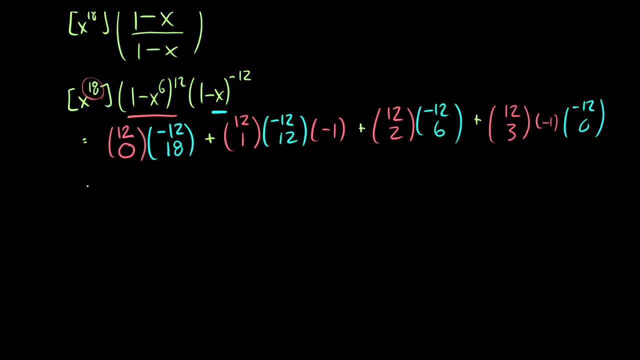 But then we'd be at x to the 24. And we can't have that. So Now We can do some simplifying. Well, 12. Choose 0. Is just 1. So we have Negative 12.. 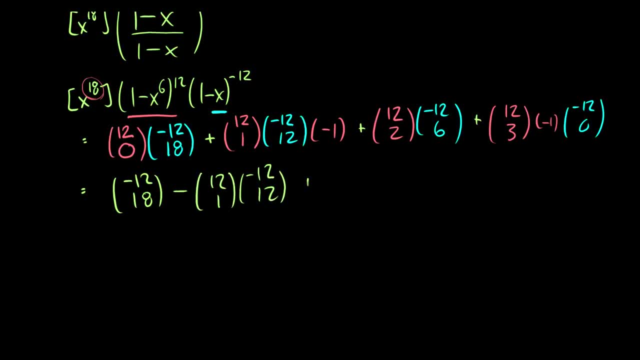 Choose 18.. We're going to subtract 12.. Choose 1. Times, 12. Choose 2.. Times Negative: 12.. Choose 6.. And then we'll subtract 12.. Choose 3. And. 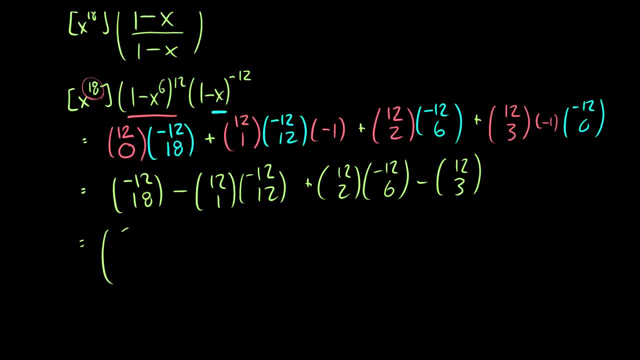 Negative: 12. Choose 0. Is just 1. So We can simplify this further. This will be 29. Choose 18. Because Negative Or Sorry: 12. Plus 18. Minus 1.. 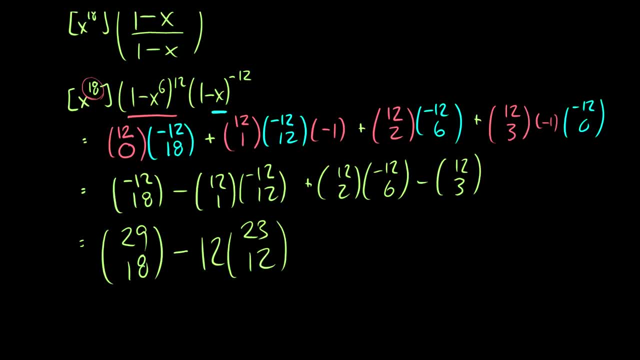 Is 29.. We'll subtract 12. Times 23. Choose 2.. Times 17. Choose 6.. And we'll just subtract 12. Choose 3.. So That would be the answer. 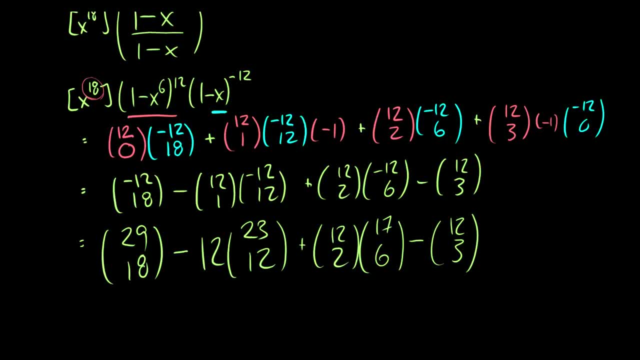 It's kind of It's kind of difficult. I know it's difficult And Originally This was a probability question, But I decided against Doing the probability version Because Really It's taking away From the Okay. 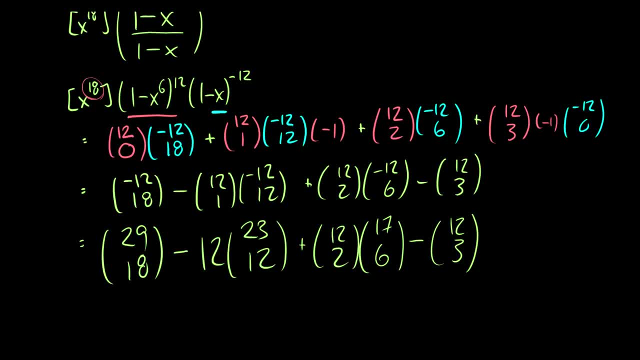 How do I do this difficult Generating function? And it's putting it More In the right place So We can. And it's putting it More into a Oh, What's the extra step here? And that's not necessary. 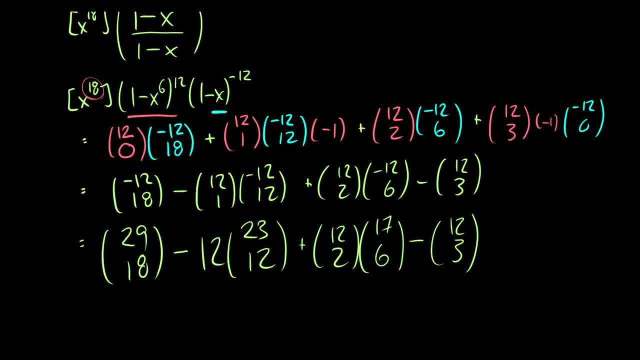 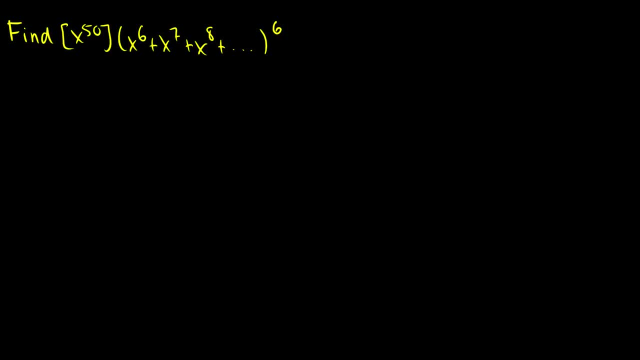 For a video On how to learn To do this stuff. So That was the Probability example. Let's do one Quick One here: Try. This is your practice, So please Do it right now If you can. 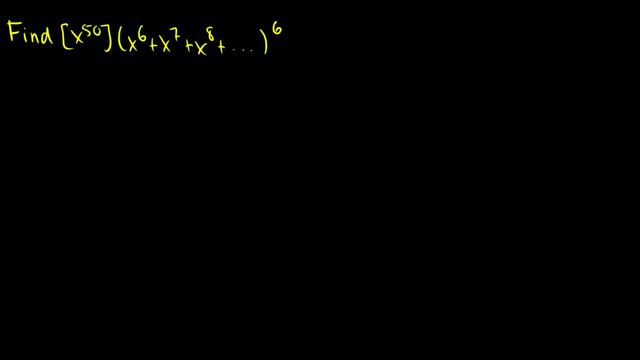 Okay, Well, You can pause the video If you want to try it. So We'll do the same thing here. We're going to take An x6.. Out of all, Six of these We're going to take, 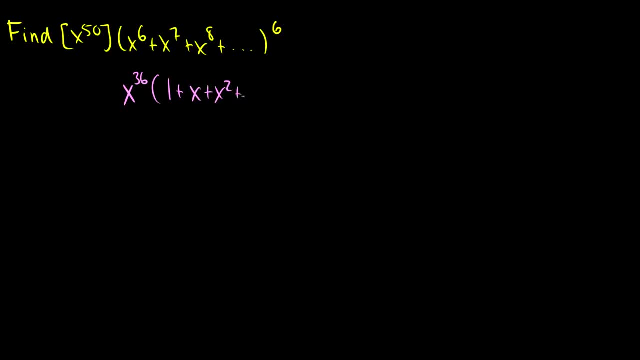 An x36. Out, And we'll be left with One plus x, Plus x, squared, Plus Dot Dot Dot. And of course We want the fiftieth Coefficient, Because this is shifted Over now. 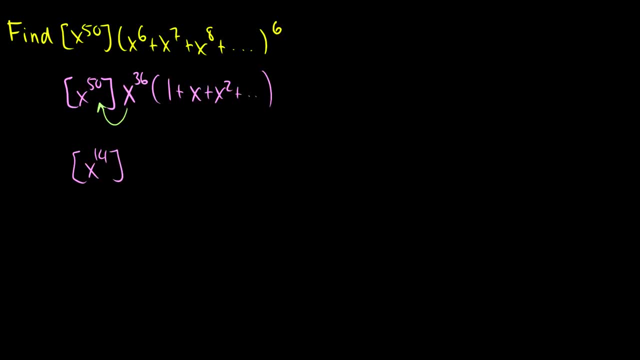 We'll just Shift it Back And we'll be left with X to the fourteen Of One plus x, Plus x, squared, Plus Dot, Dot, Dot. And This is You know The mean Of.